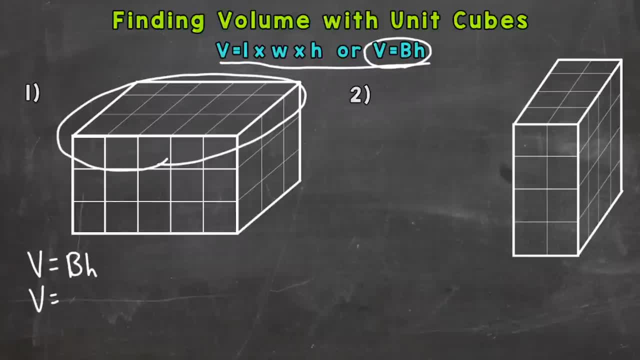 or area of one of the layers is 15.. Now we can find the volume or how many unit cubes take up that shape by multiplying one layer by how many layers there are- And there's one, two, three layers- 15 times 3, so we could do 15 times 3, and that will give us how many unit cubes make up. 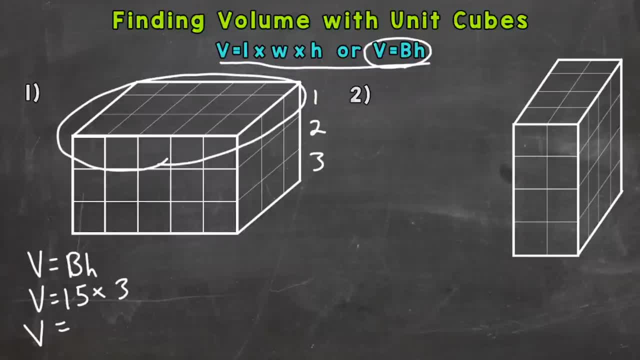 that rectangular prism, and I will put Cu, which means cubic units, and that's the volume of that rectangular prism, And volume is how much space a three dimensional object takes up, undefined. Let's use our other formula: 10 times 3,. 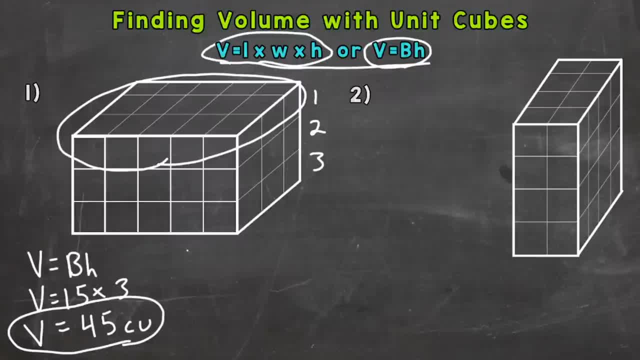 and see if we get the same answer. Volume equals length times width, times height. So length, I consider how far back the three-dimensional object goes. So if we take a look here, how many cubes back? Well, three times the width. How wide Five. 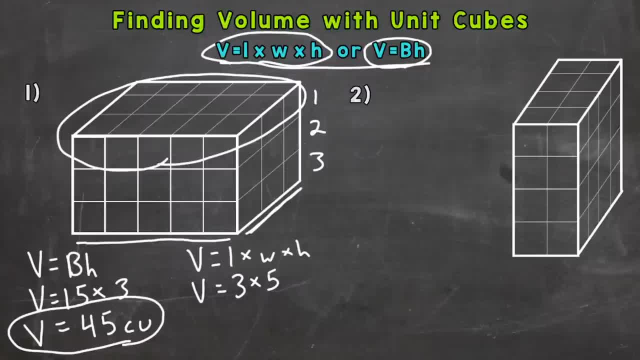 unit cubes And lastly, how tall the height. Three unit cubes- And this will get to 3 times 5- is 15, times that 3 gives us 45 cubic units. So both formulas give us the same answer And that will happen for every rectangular prism Again. 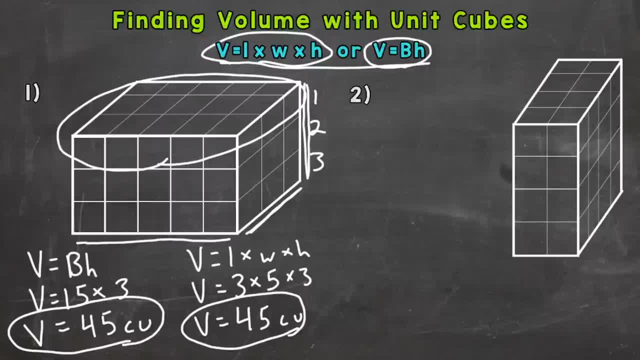 volume is how much space a three-dimensional object takes up, and volume is how much space a three-dimensional object takes up. and volume is how much space a three-dimensional object takes up, and we use unit cubes in order to measure that space, whether it's cubic inches. 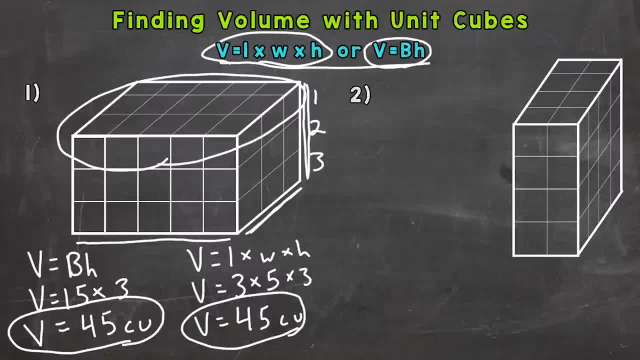 cubic feet, cubic yards, meters- Here we're just using cubic units. the unit of measure is not given. So let's take a look at number two. So we have a rectangular prism there. We're going to find out the volume by finding how many. 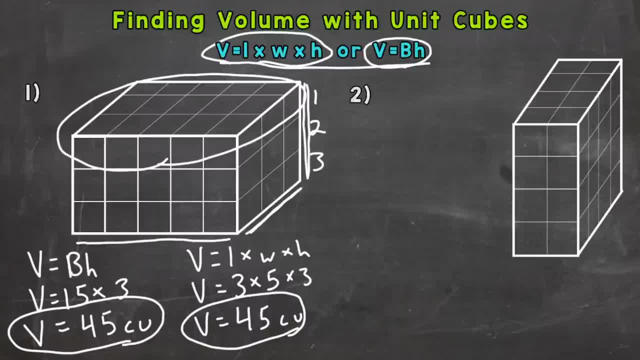 cubic units fill that rectangular prism. So again, two formulas we can use. We'll go through both. Volume equals the area of the base times the height. So for this one, you find the area of one of the layers and then multiply it by how many layers there are. So let's take a look at the top. 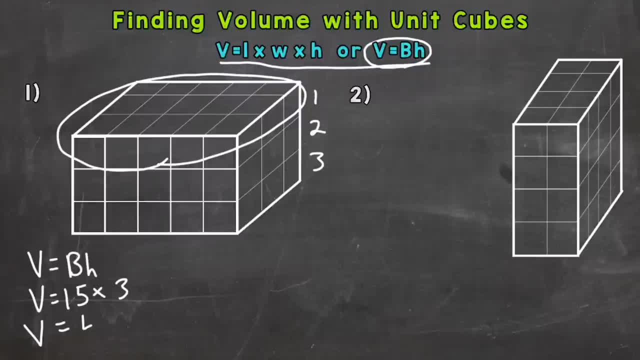 prism, And 15 times three gives us 45.. And I will put Cu, which means cubic units, And that's the volume of that rectangular prism And volume is how much space a three-dimensional object takes up. Let's use our other. 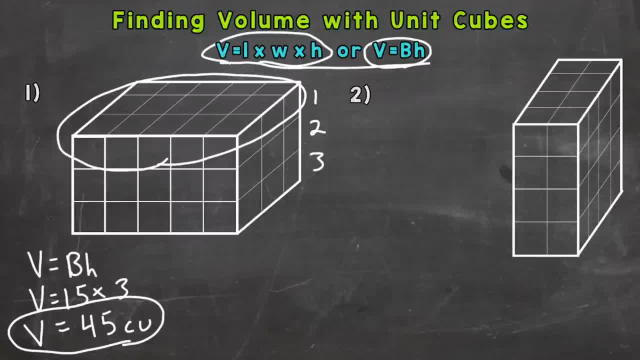 formula and see if we get the same answer. Volume equals length times width, times height. So length, I consider how far back the three-dimensional object goes. So if we take a look here, how many cubes back? Well, three times the width. How wide Five unit cubes? And lastly, 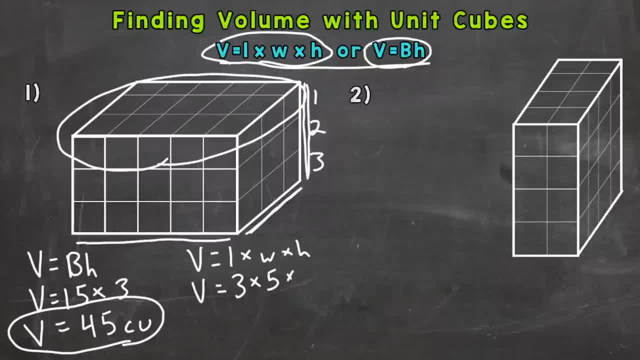 how tall the height. Three unit cubes, And this will get to three times five, is 15 times that three gives us 45 cubic units. So both formulas give us the same answer And that will happen for every rectangular prism. Again, volume. 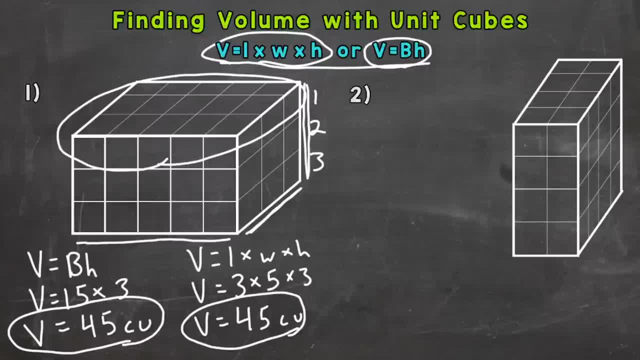 is how much space a three-dimensional object takes up, And we use unit cubes measure that space, whether it's cubic inches, cubic feet, cubic yards, meters. Here we're just using cubic units. the unit of measure is not given. So let's take a look at number two. 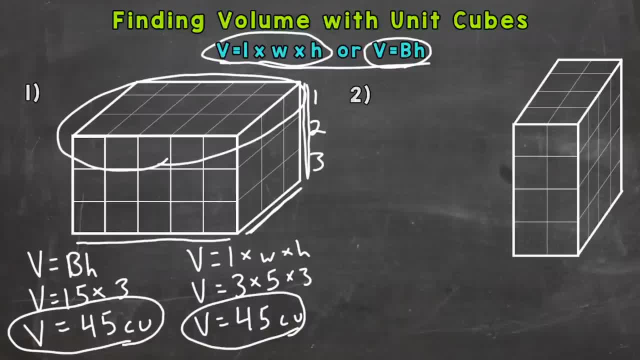 So we have a rectangular prism there. We're going to find out the volume by finding how many cubic units fill that rectangular prism. So again, two formulas we can use. we'll go through both. Volume equals the area of the base times the height. 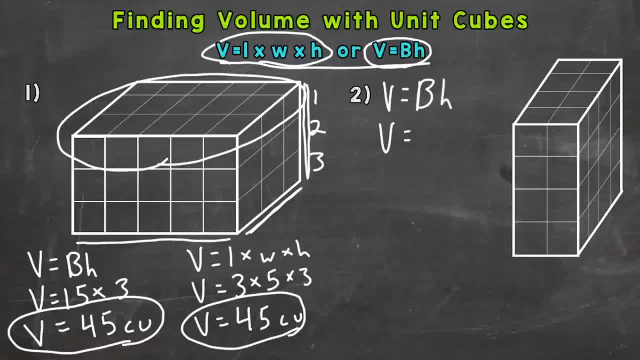 So for this one, you find the area of one of the layers and then multiply it by how many layers there are. So let's take a look at the top layer. How many unit cubes make up that top layer? Hopefully you're thinking eight.